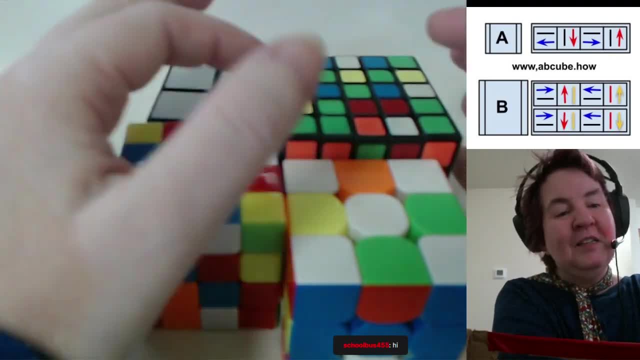 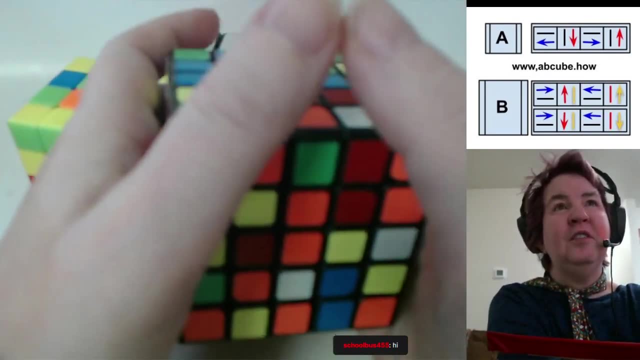 So formula A is 4 moves, And it's one row, one column, And just like B, it's a mathematical zero, It's a commutator: For every left there's a right, For every up there's a down. 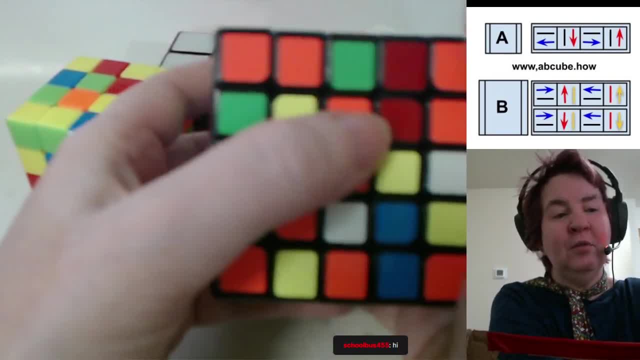 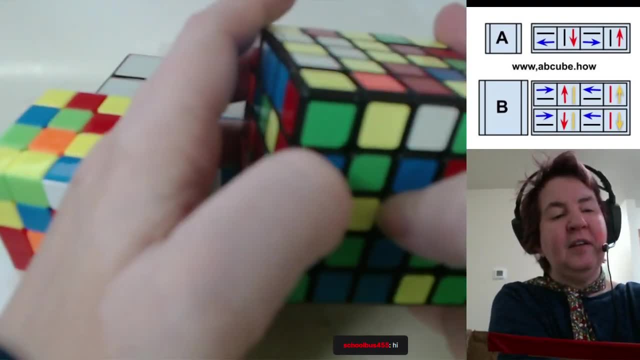 So it doesn't move. It only moves the pieces that you want to move. It doesn't mess up the rest of the things you've already solved. So formula A can affect the absolute center, Or it's usually done to affect the corners. 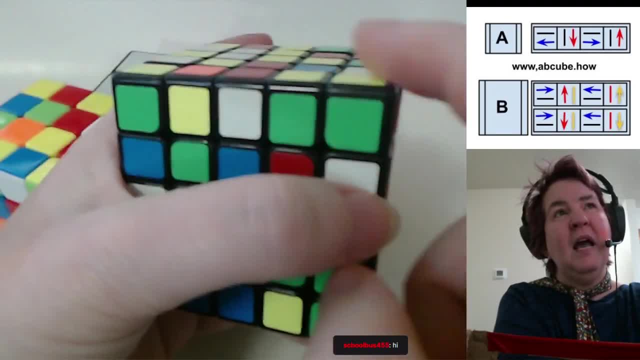 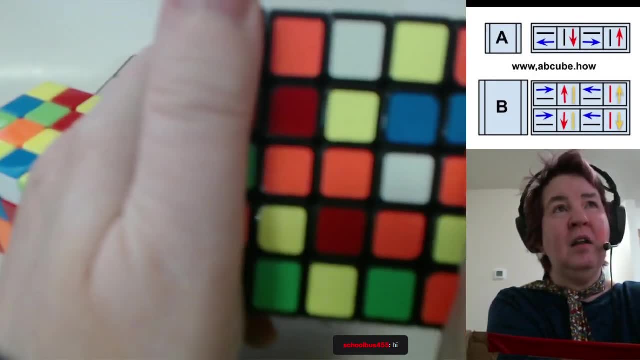 Bottom row, right column. It'll bring a corner to the top And it'll twist the corner around If the corner needs to twist. That's formula A. Formula B is the top row and two columns, And depending on which two columns you use, you select the piece you want to move. 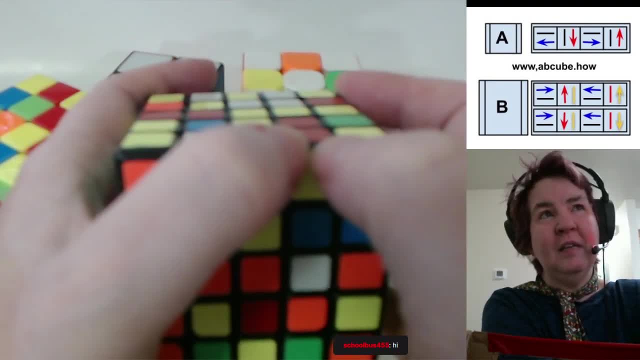 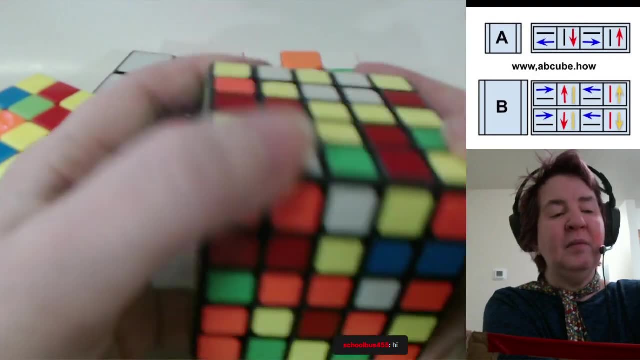 And the two columns are determined by the cube, based on where that cube is to begin with and where that cube wants to land. So formula A with the formula B with the outside columns, moves corners Outside, inside, one outside, one inside moves edges. 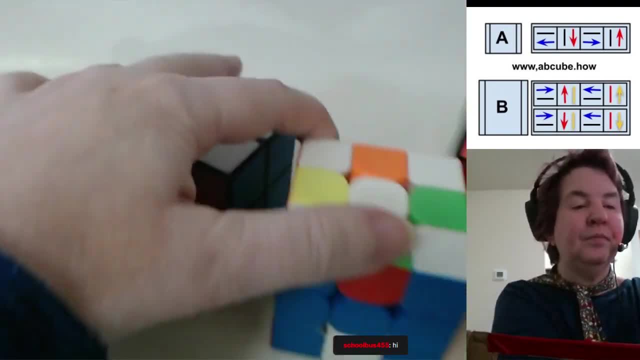 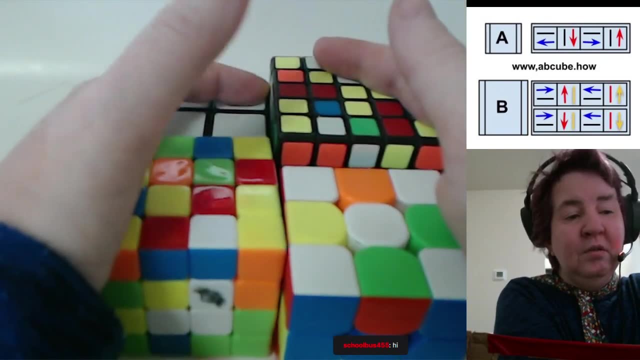 And two inside columns will move sides. So that's formula A And with formula, with that, that and formula A is all you need to do, all you need to know to learn in order to solve every complexity. Rubik's cube. 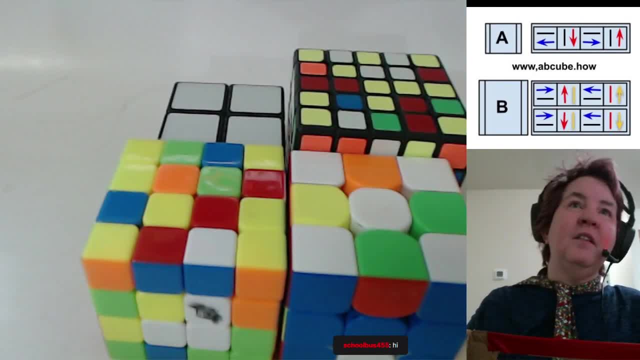 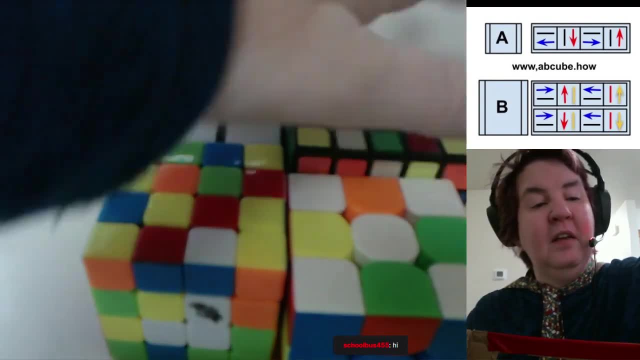 But it, like I said, it is not a speed solve method, It is not a few smooth method, But you can learn the inside of two hours And it apply it to every complexity cube. So you can, you can. when I teach the cube, I teach starting with. 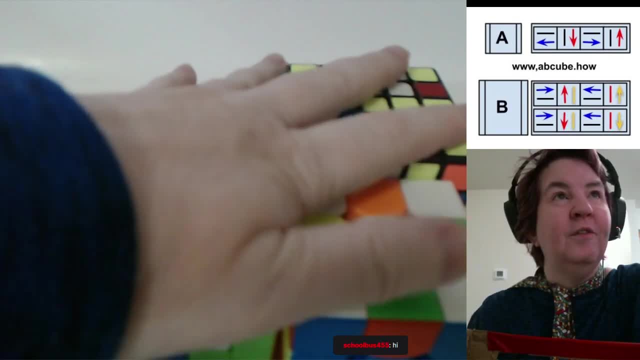 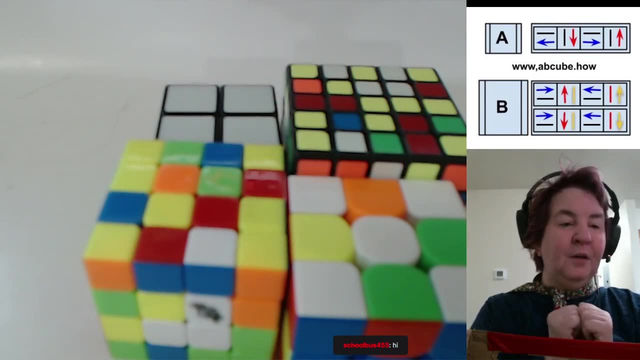 either the five by five or the four, the four set of learning cubes: The two, three, four and five. So, that being said, who do we have with us today? I always feel like Romper when I stream, Okay. 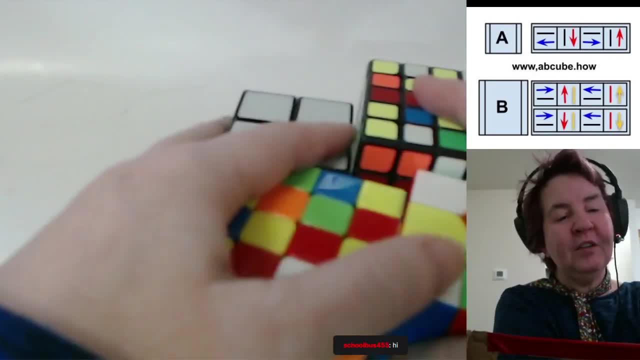 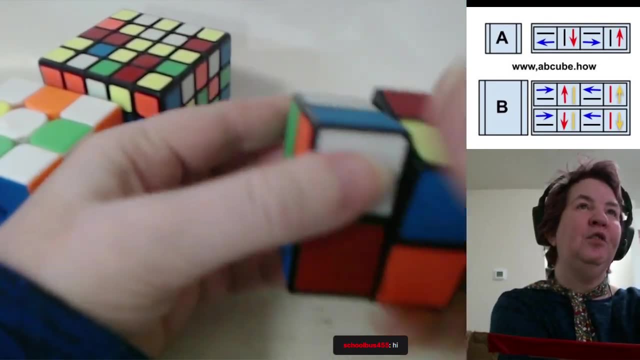 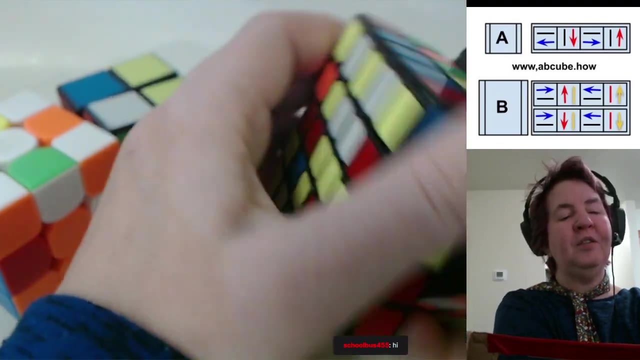 All right, So I have did the corners on Saturday. I'm going to scramble them all. Monday is a good time to start with corners. Okay, So, no matter which cube you have in your hand, that cube has eight corners. 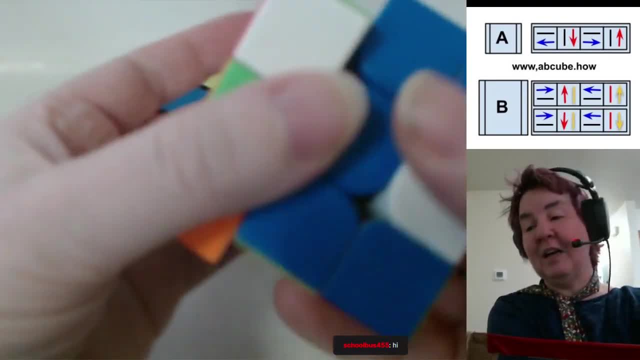 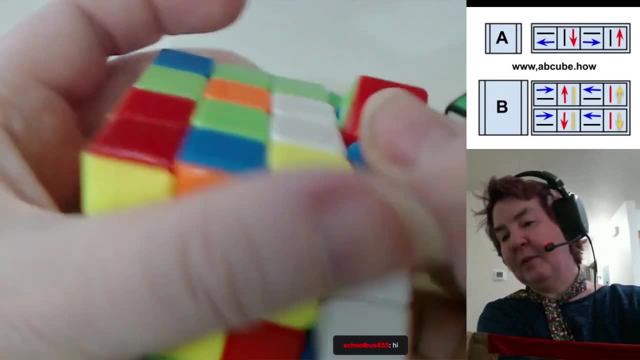 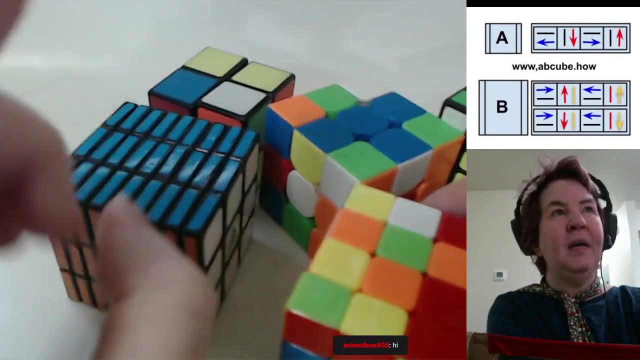 This it will work on. it will work on anything that is an n by n by n cube. It will work on some of the work on the three by nine. we need a three by nine with a minor adaptation. It works on some shape mods. 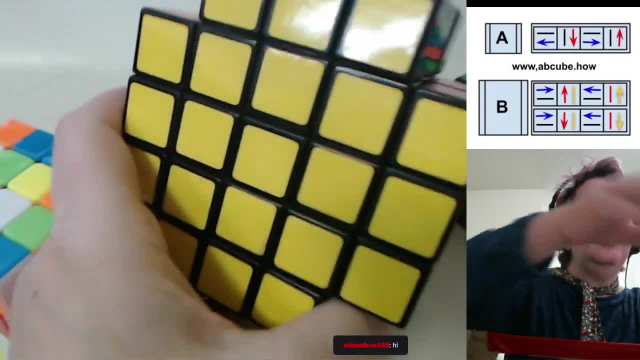 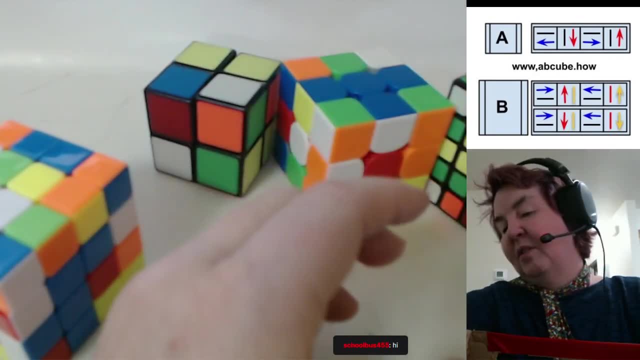 And I can solve this five by five, this plus cube with it. Just pretend that it's a five by five cube with pieces missing And work with the columns that are left. It also works on every minx. It does not address parodies. 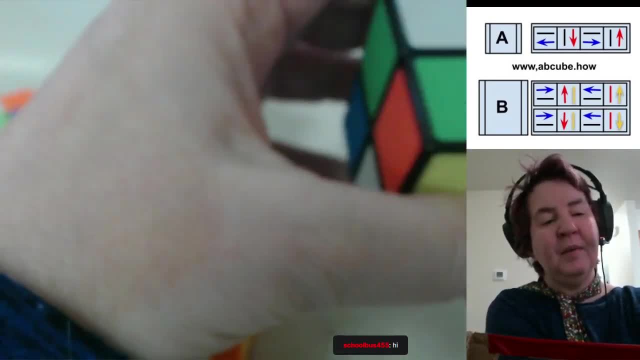 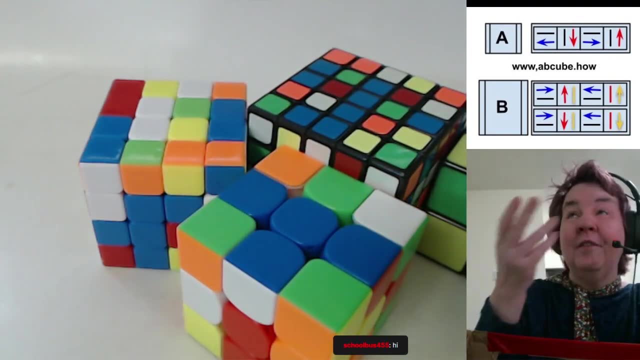 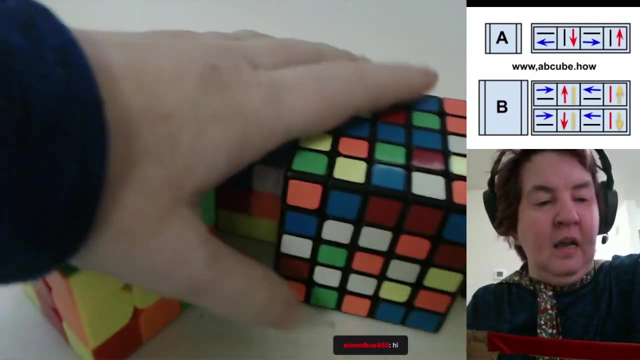 It's because parodies are a lie And you don't have to play with them unless you want to, Because, like I said, formula A brings a piece to the top And formula B moves three pieces around, And with that you can solve every complexity. cube. 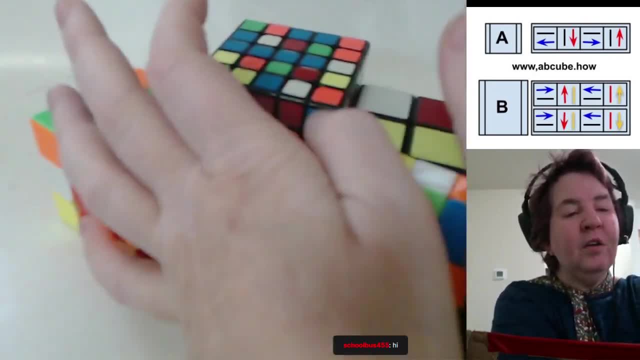 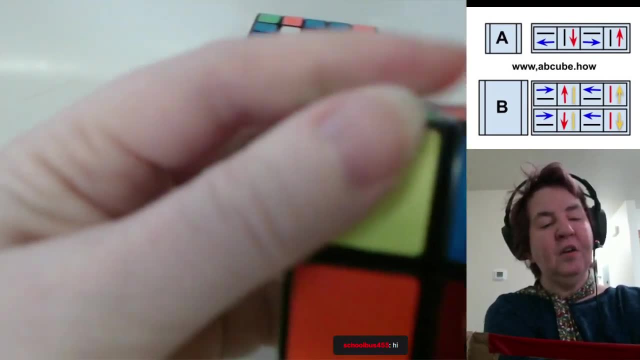 So your cube has eight corners. Pick a corner. Your corner has three colors on it. Pick a color. We're going to start by working with just the corners And we're going to start with working with just one color, And so I start with yellow. 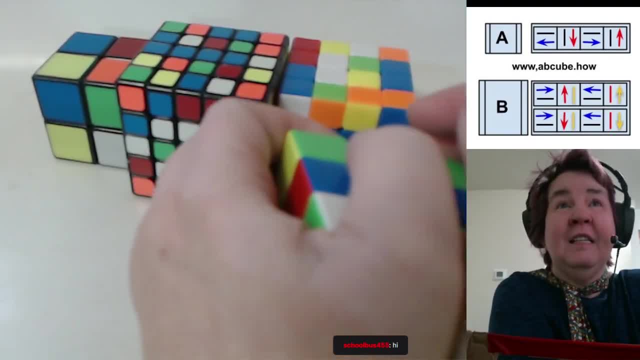 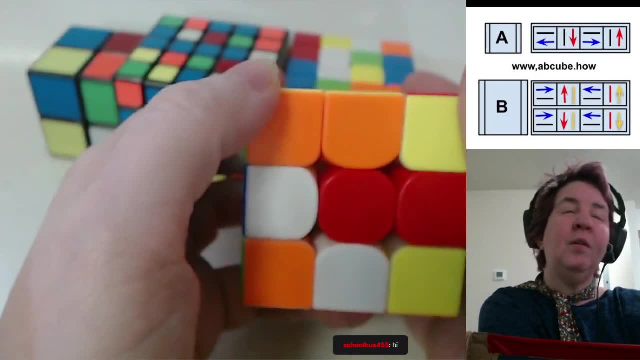 Because I was color neutral and my alpha tester said: tell us what to do. So okay. So I find a corner piece that has a yellow on it. I put it under my left thumb. I'm holding it in both hands. 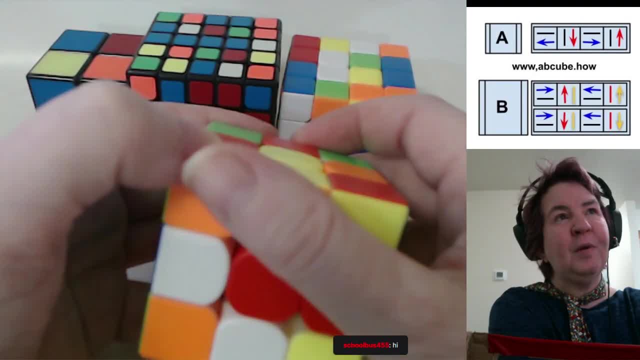 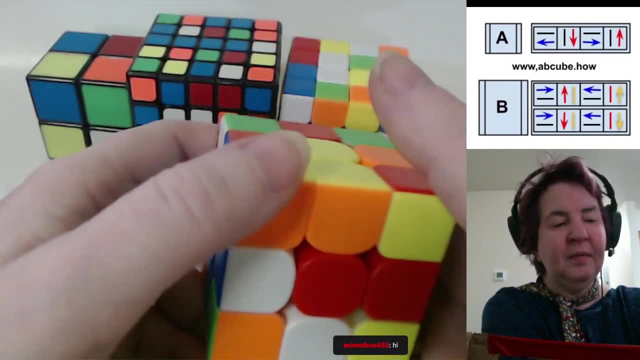 And again, I'm looking at the front of the cube as if it were a spreadsheet with rows and columns. So the corner that I selected is under my left thumb With the yellow, with the active color on top. This corner, then, is correct. 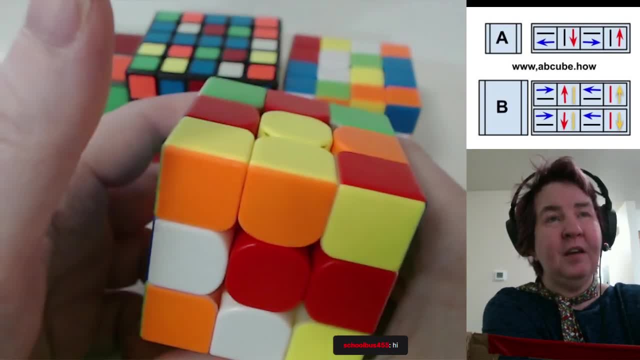 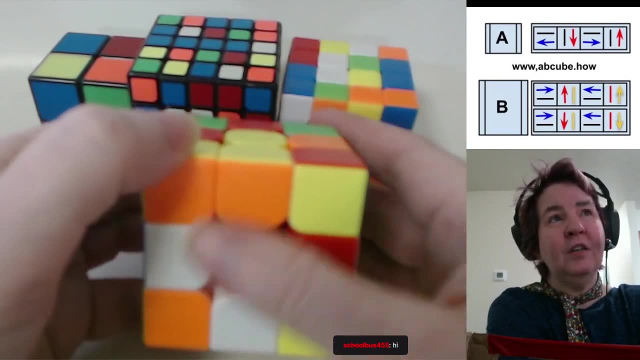 We're going to make all the rest of the cube match it, Because that's how powerful you are. The cube that you select is the right one. So we're looking at only corners. So we look at the corner that's under my right thumb. 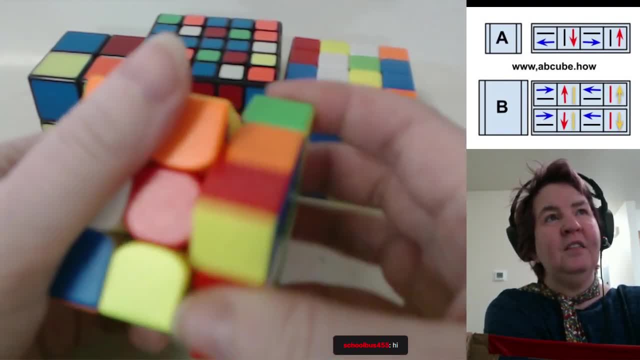 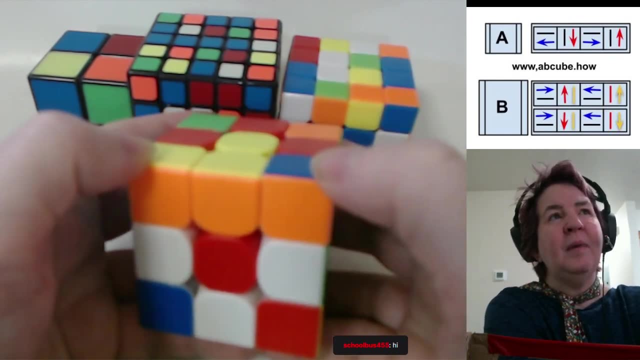 Now let's see. This looks too simple. I didn't scramble it very well. It's making it more messy. Okay, So we look at the corner under my right thumb, Because the left one is correct. We're going to try to match it. 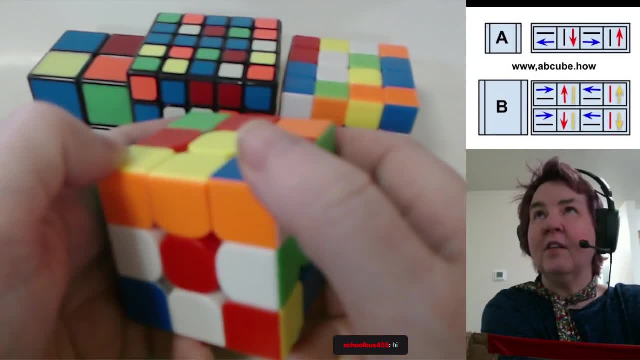 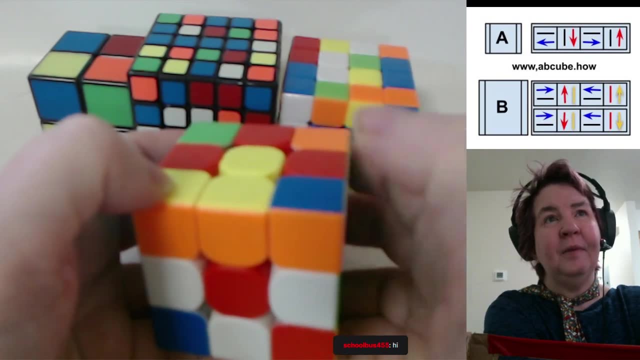 So we look at this corner and we see our active color is yellow. So we're looking to see if there's a yellow anywhere on these three corners And if there is, is it on top? If it's on top, we're going to slide it out of the way. 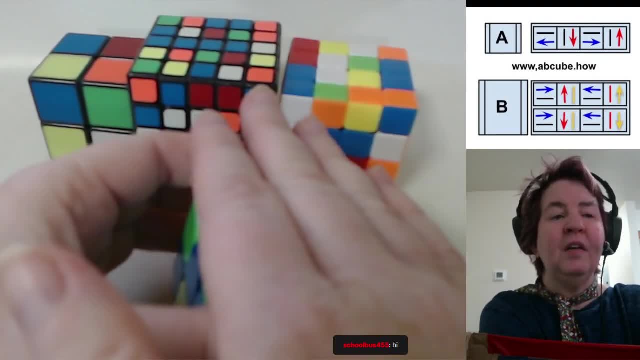 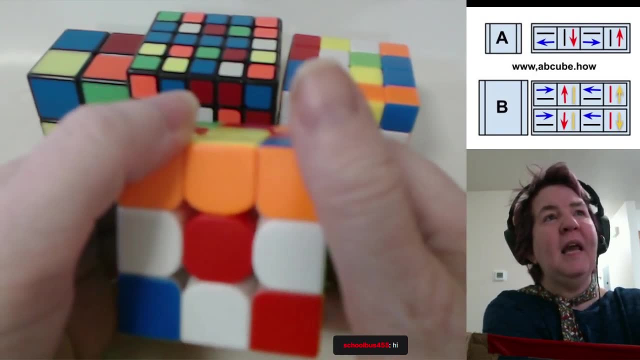 and keep going with the next corner. So the first thing we're going to do is we're going to bring yellow to the top on all of our four corners. So if there's a yellow anywhere here, formula A will bring it to the top. 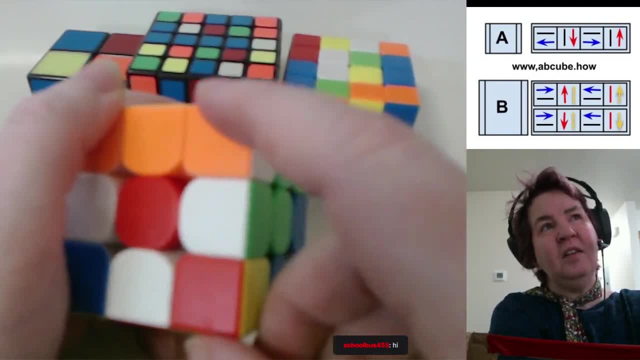 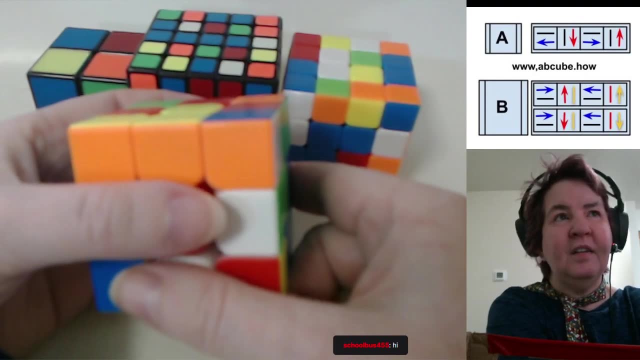 If there's not, we look down here at this, The other corner, Because these are the two corners that are going to flip back and forth. So if there's yellow anywhere here or here, then formula A will bring it to the top. 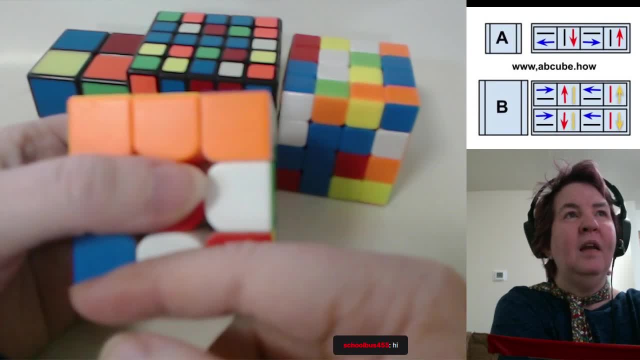 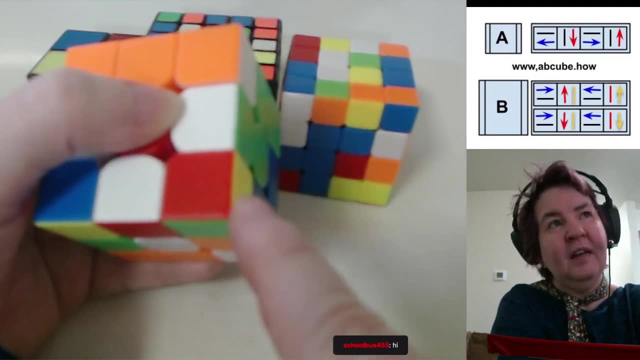 So one row, one column. It's the bottom row and the right column, because I'm right-handed, So the action is taking place in this row. So I want to preserve this piece, So I'm going to move it out of the action. 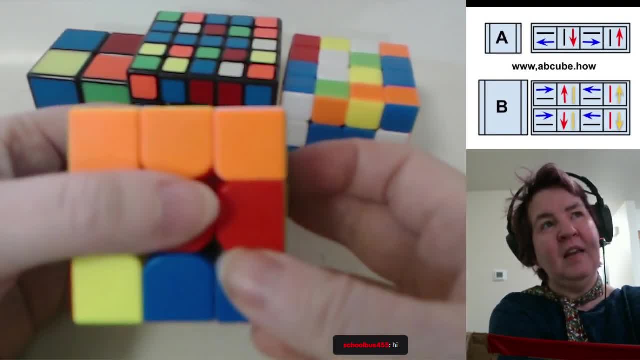 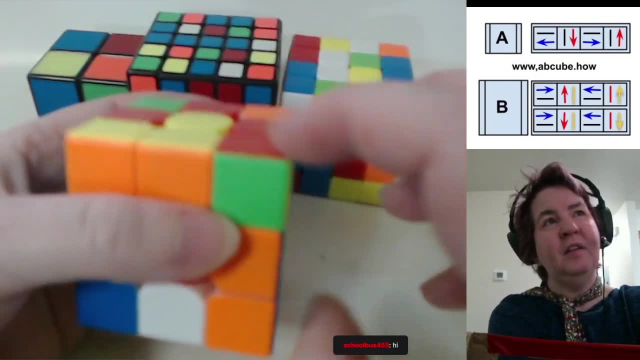 Away from the action. Move the space down, Move the cube into the space And the cube moves space back up again. So that flipped. these two Did a bunch of other things, but we don't care about that yet. So is yellow on top. 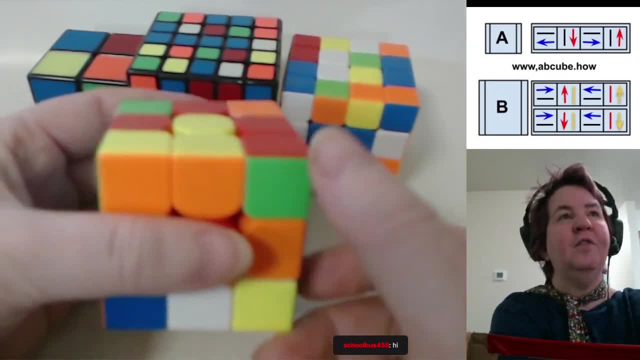 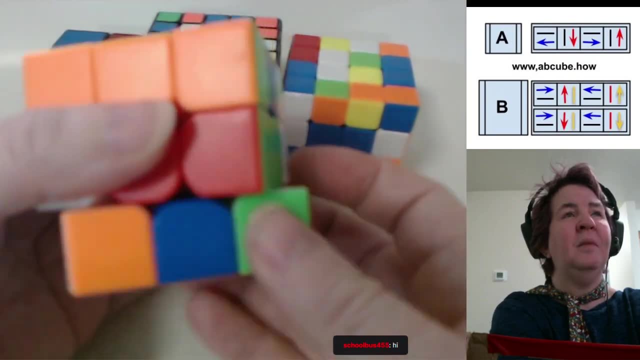 It's on the top layer but not the top face. So I'm going to do formula A again And I'm going to keep doing formula A until the yellow does come to the top face, Because it will. And when it's on the top face, 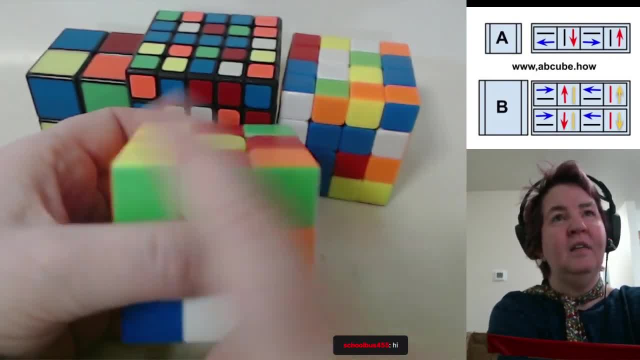 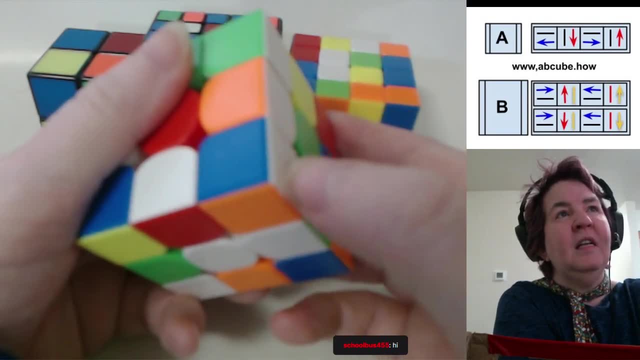 then I hold the cube stable, Slide the top out of the way to protect it, And I keep going. So is there a yellow anywhere on this cube? No, Is there a yellow anywhere on this cube? Again, if there's a yellow anywhere on these two cubies, 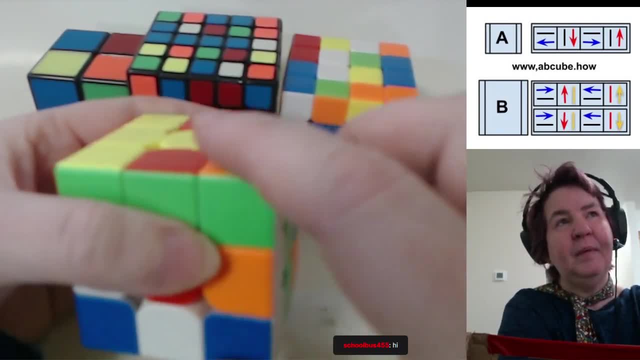 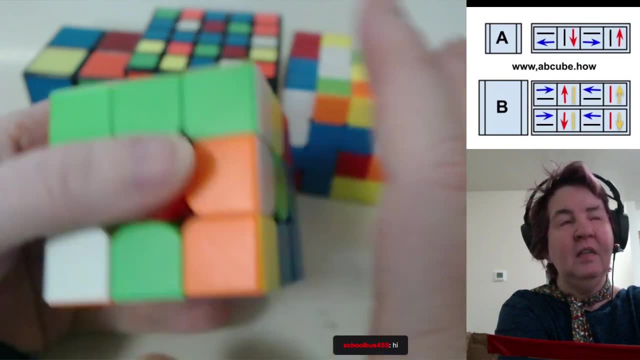 these two corner cubies. A will bring it to the top because it switches these two and twists them around. But if there's not, you have to rotate the bottom by quarter turns to keep the cube stable. Rotate the bottom by quarter turns until the answer is yes. 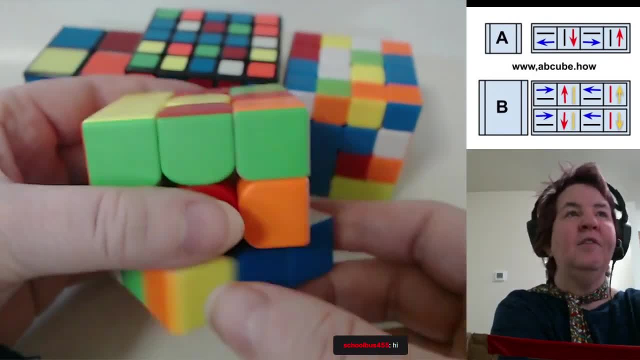 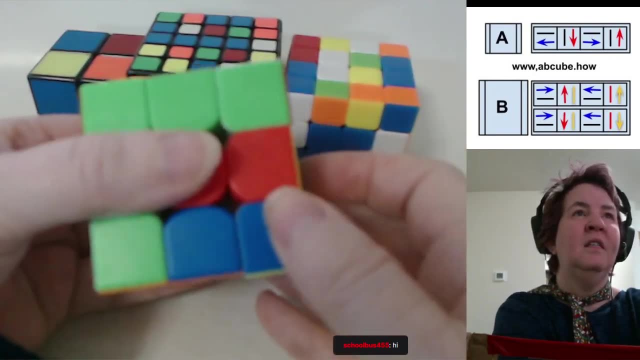 So there is a yes, a yellow on one of these two And formula A will bring it to the top. It doesn't do it right away, We just keep doing it. There are again. there are shorter ways, There are quicker ways. 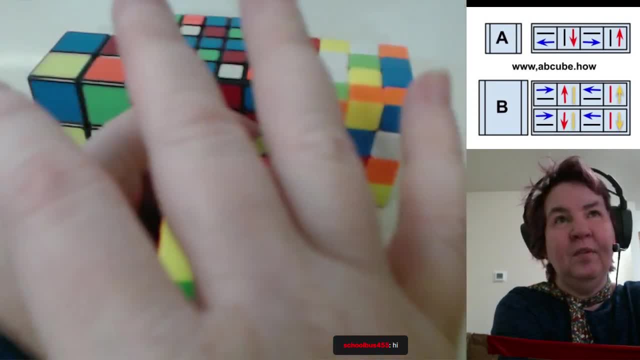 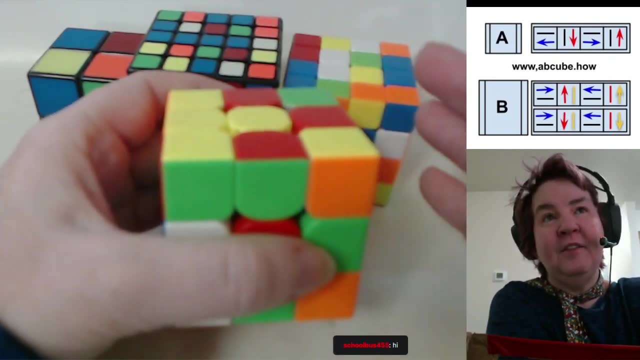 But this is, this is. this is a I teach total non-cubers who think they can't learn inside of ten minutes, inside of two hours. So yellow is on top, Hold the cube stable, Slide it out of the way. 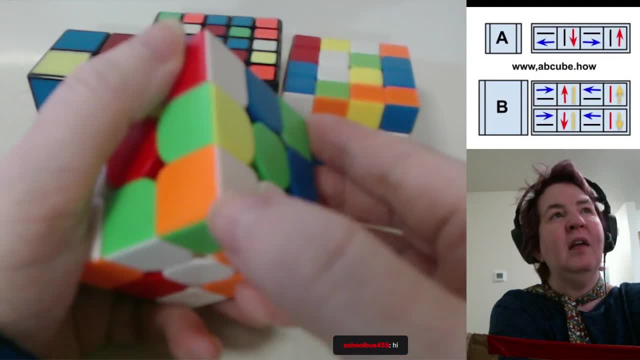 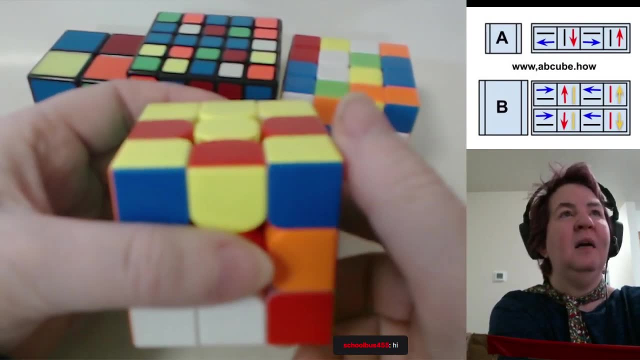 Keep going with this cube. If there's a yellow here or here, A will bring it to the top. If not, I rotate the bottom until there is And then out down. in up Yellow is on top on all four corners. 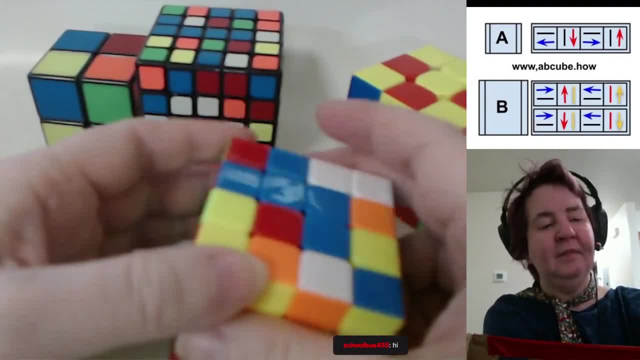 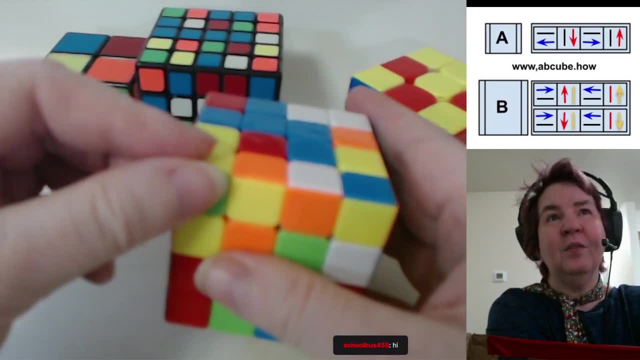 That's what we wanted to do, So let's do that again. One, the we find the yellow And that's our. that's. that's. this is the correct corner. We're going to make all the rest of the cube match it. 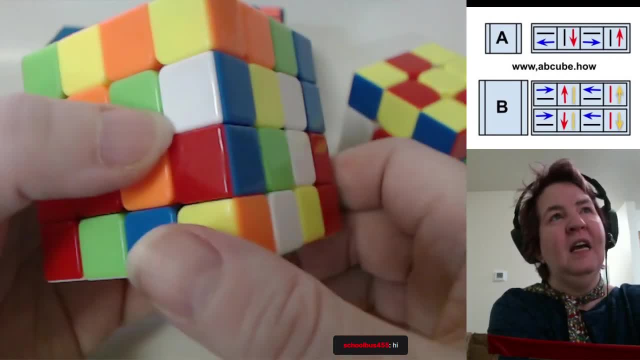 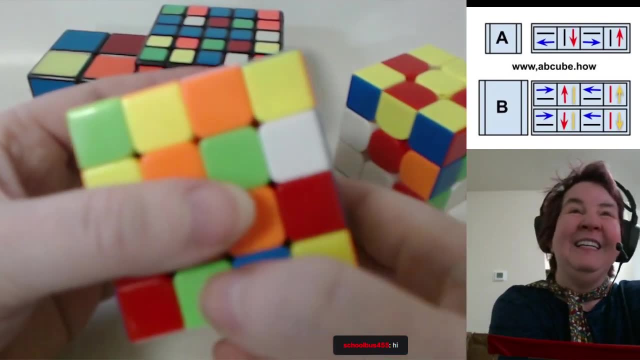 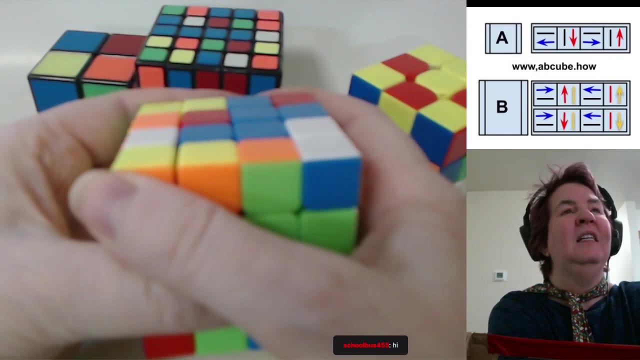 So is there a yellow here or here? The answer is yes. I can muscle it into place, But I don't want to do that because it of it out down in up. Okay, Slide, Keep going for corner. yellow here or here? 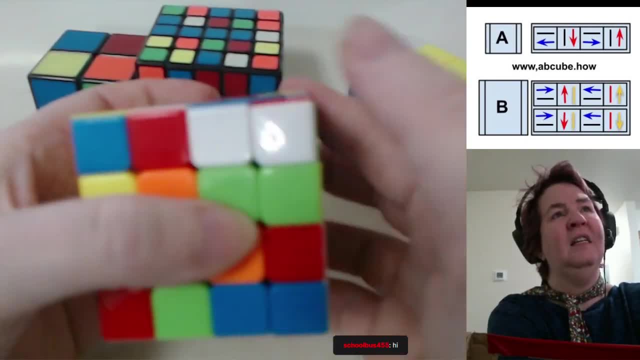 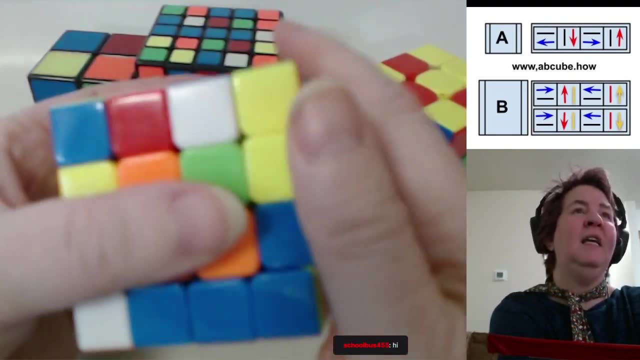 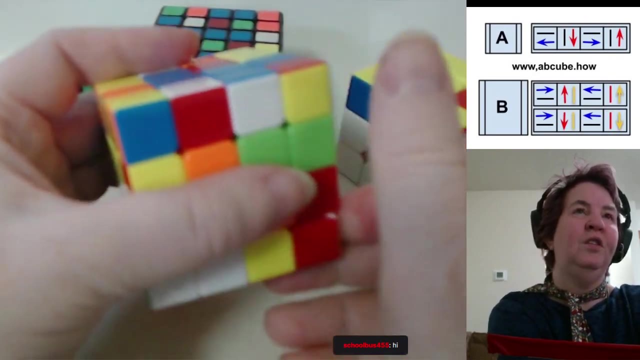 Out down in up Slide, Keep going. Is there a yellow here or here? No, Rotate the bottom, There it is, And then formula A will bring it to the top In five or less moves. All right, 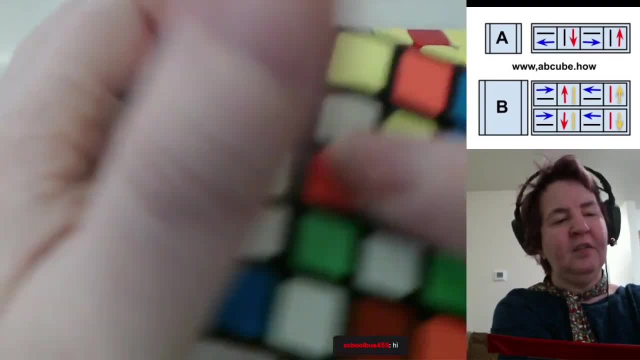 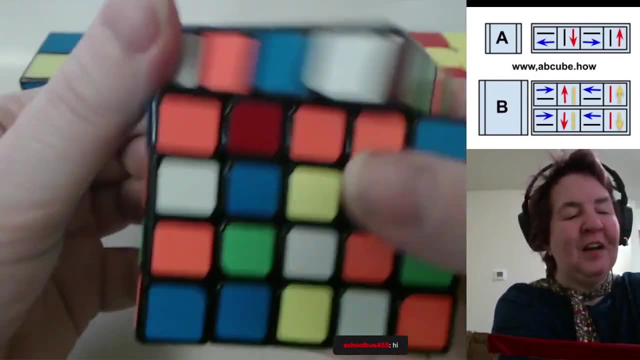 So yellow is on top on all of these. Let's try this one. I didn't scramble this one yet. Ha ha, ha, It's still solved. Corners are solved from yesterday, from Saturday, Let's just scramble. 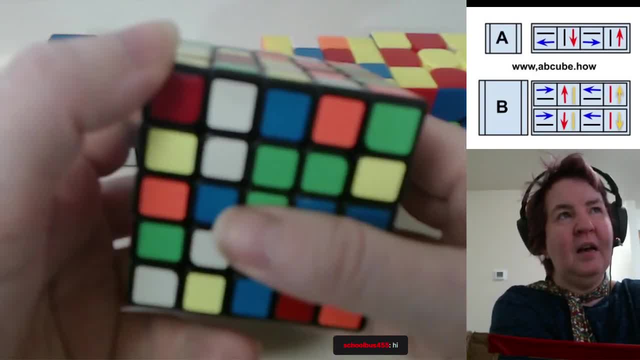 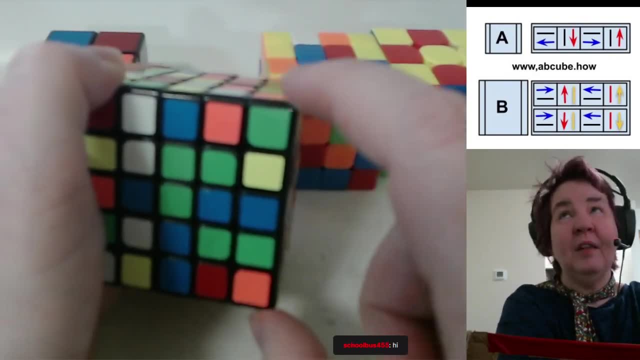 Okay, Find a corner that has yellow on it. It's on the top face and it's under my left thumb. I look at this corner. There's no yellow, but there's a yellow on this one. So if there's a yellow on one of these two, 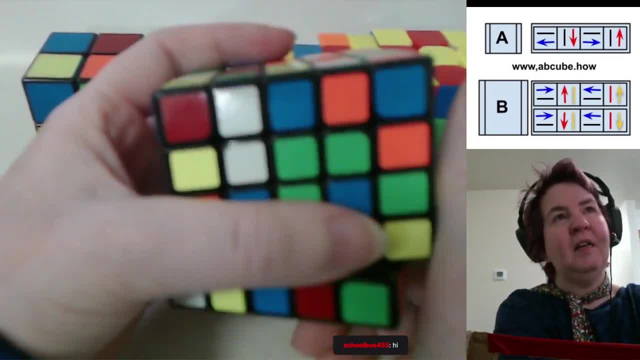 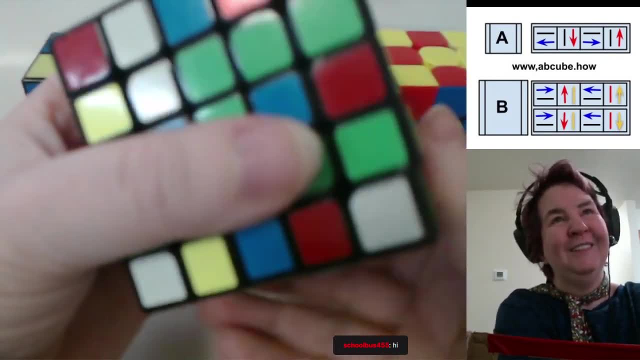 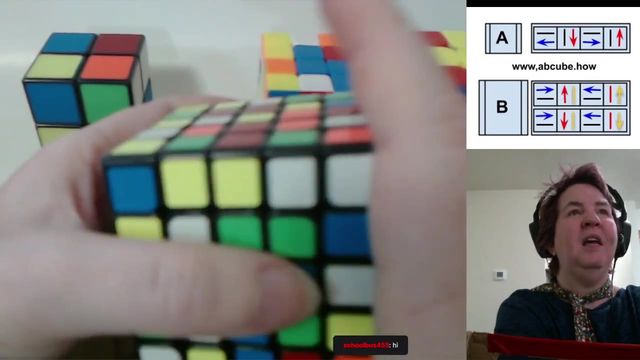 formula A will bring it to the top Bottom row right column And when it's on top, slide the top to protect it, Keep the cube stable and continue if there's a yellow here or here And if not, now there is. 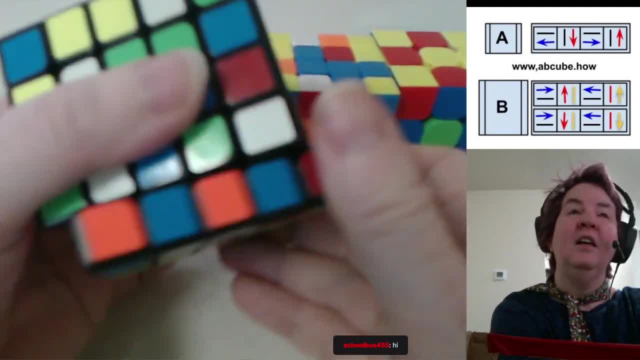 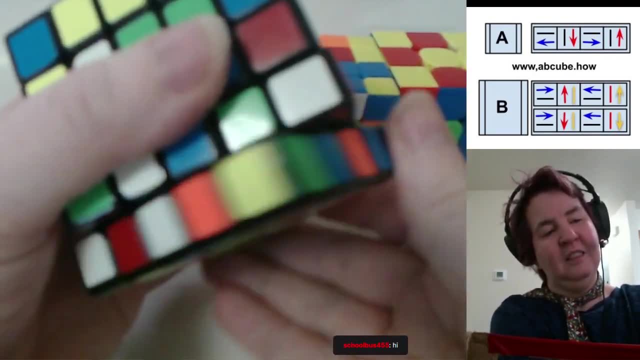 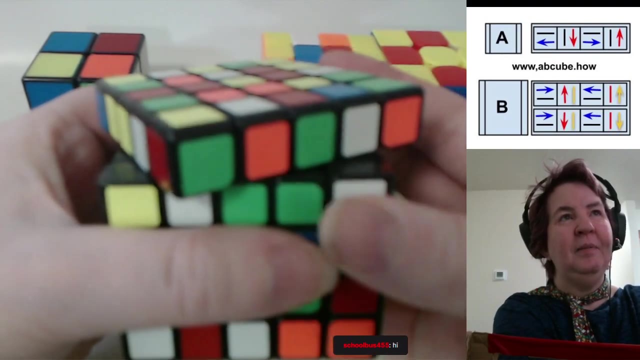 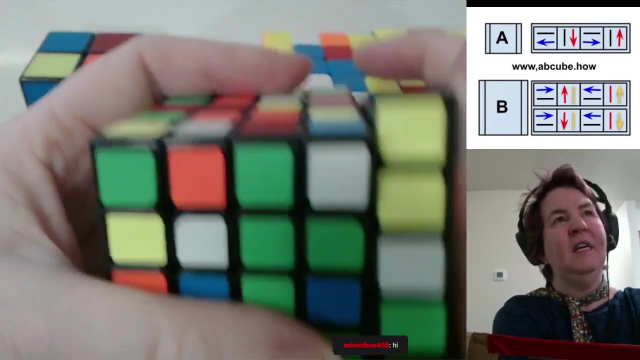 So formula A will bring it to the top. Okay, And yellow is on top. Keep the cube stable, Slide the top to move it out of the way and continue with this corner. There is a yellow Out down in up. 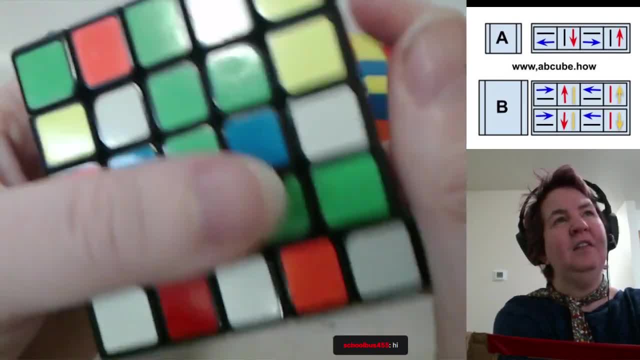 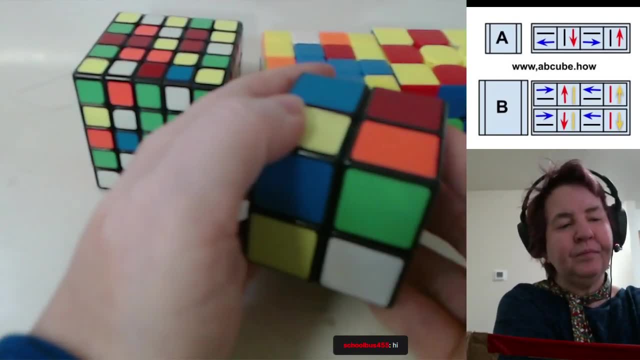 Out, down in up, Out, down in up, And there it is. Yellow is on top. Okay, Let's do it again. Is there a yellow here or here? No, There's a yellow there, Okay. 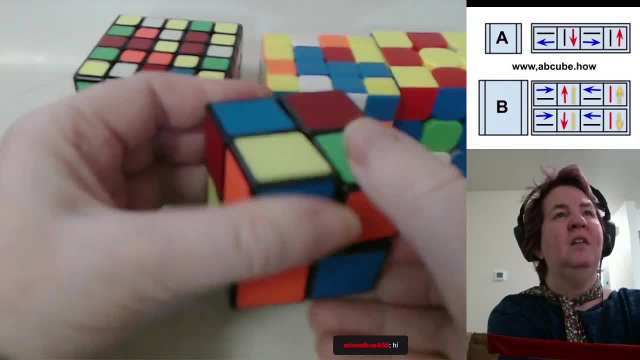 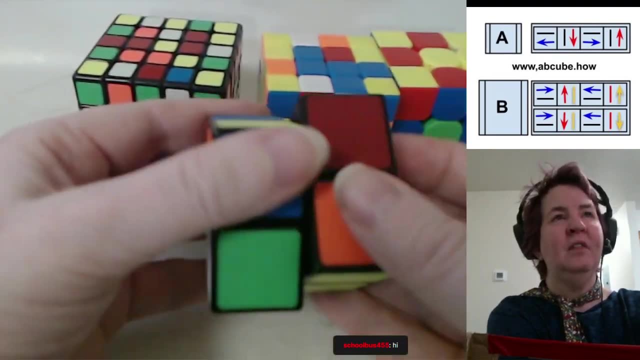 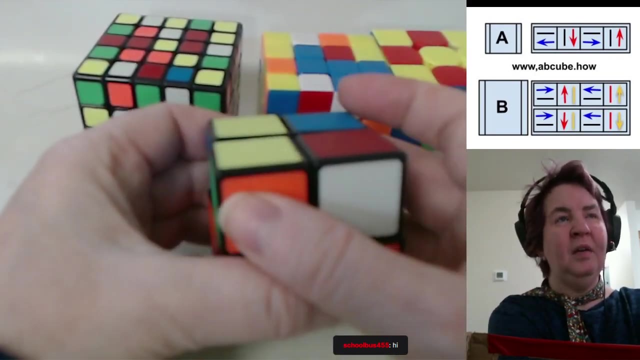 So formula A will bring it to the top Bottom row, right column. For every left, there's a right. For every up, there's a down. Okay, Slide the top. Keep the cube stable. Slide the top to protect it. 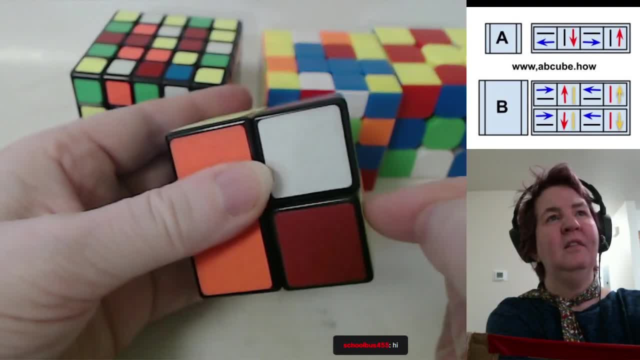 Is there a yellow here or here? No, But there's one there Now. there is Out down, in up. Until the yellow comes to the top, There it is. Slide it out of the way, Keep going. 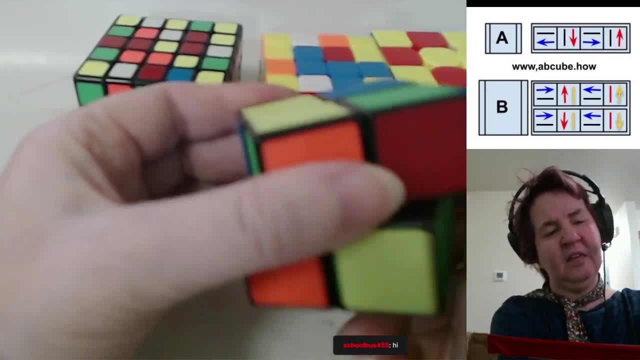 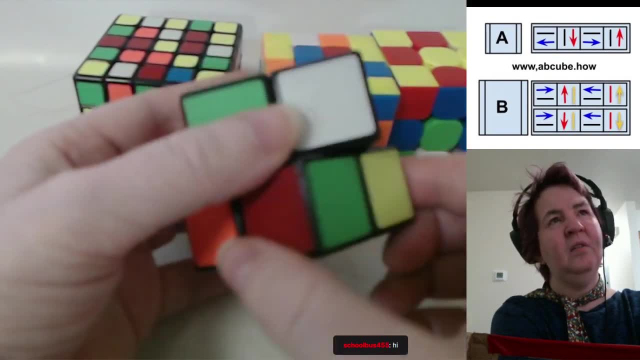 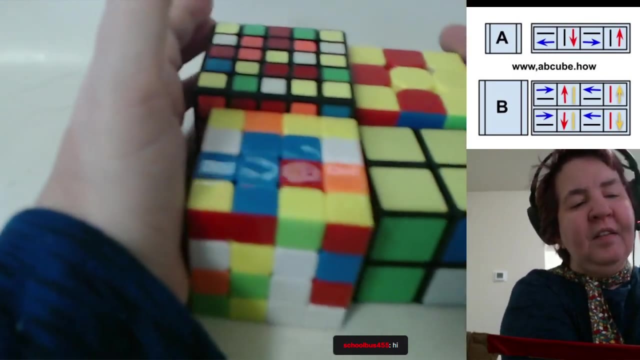 Yellow here No, Yellow here No. Now there is Out down, in up Yellow's on top of all four corners. Okay, So when you get to this point, one of three things has happened Because your corners, your corners, are not aligned. 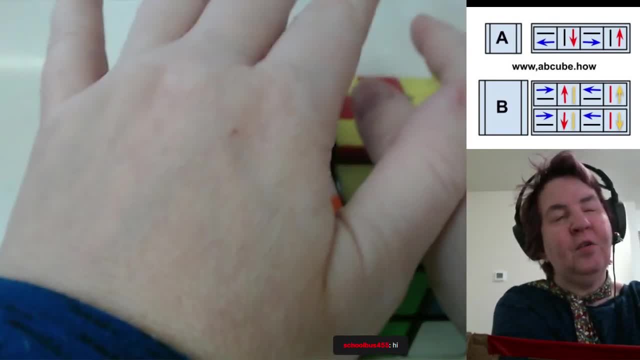 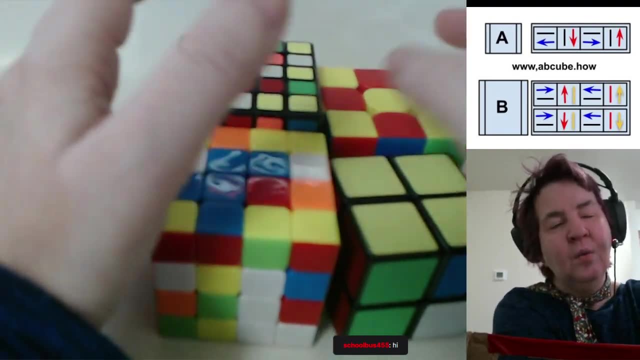 They're not aligned. Okay, So what's the problem? Because your corners, your corners, have three colors and not just one, So the yellow with the active color on top, in this case, yellow. we're now going to look. 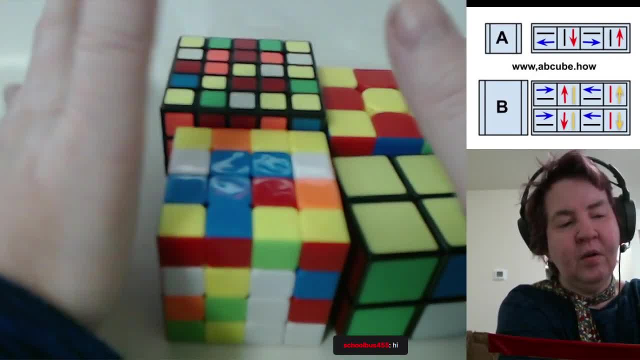 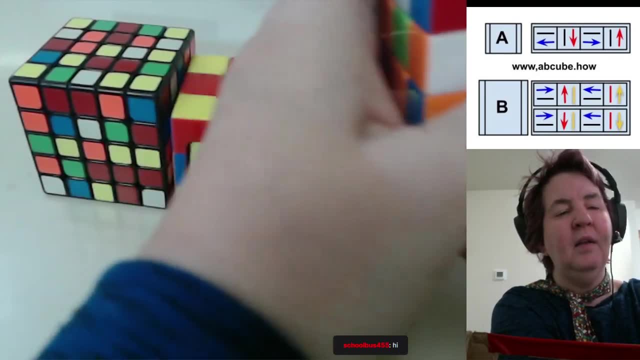 at the other two colors of the corners, We're still ignoring everything but the corners. We're only looking at the corners, And but instead of looking only at yellow, we're looking at the other faces as well. So, at this point in time, one of three things has happened. Either the sides keep the cube stable. Now, the reason why we're keeping the cube stable is because It really doesn't matter at first, Is because we will solve the second four corners the exact same way we solved the first four corners. So you only need to learn one way to solve the corners, because it works on the first and the second. The first four and the second four. So yellow's back to the top and the corners match. Okay, Again, matching color behind. We're ignoring everything but the corners. And then formula B- Slide up, Slide up, Slide down, Slide up, Slide down, Slide up, Slide down. And then this one stayed the same. These three all moved Formula B, A formula to bring the cube, the color, back to the top. Keep the cube stable. The reason why we're keeping the cube stable is when we're working on the second four corners. if we rotate the cube while we're in the middle of a set, it will scramble the rest of the cube. We don't want to scramble the rest of the cube. So we just learn to do it right the first time. So yellow's on top Corners match to each other, And that's the first step. But we're going. the first four corners are done. Now we're going to do the second four corners. And we do it the exact same way we did. We take the cube. Our yellows are correct. We're going to put them face down. We're going to abandon the yellows because we trust them. Specifically, what that means is: formula A and formula B is only going to affect the top layer, And so the rest of the cube will be unaffected. So these bottom four corners are going to be unaffected. So the first thing to do is: what color is opposite? yellow, because that's the color that we're going to be working on next. And so you look at the corners to see what color they all have in common. On most cubes, opposite yellow is going to be white. Some cubes are differently colored, So, but it's all. four colors have the same color And it's not a color that's touching your yellow. So it's white. If we have a white corner up already, we'll start with that one, But if we don't, it doesn't matter, We'll start anywhere, And so we're going to once we start. we're not going to twist the cube until our active color which is now white, is going to be on top, So we don't have to check to see if the white's there. We already just did that. So we know that formula A is going to bring the white to the top. So bottom row right. So bottom row right. column: Out down in up. formula A: Out down in up, And we're going to do this until the white is on the top face. There it is. Okay, Keep the cube stable, Rotate the top to preserve that And continue with this corner. Is the white on top? If so, slide it. If not, twist it until the white's on top, with formula A Out down in up. Out down in up, Out down in up. Okay, White's on top, Slide it. Keep going Out down in up, Out down in up. Slide Out down in up. Now we can see that the yellow is dancing all around, But we're ignoring it because once the white's on top on all four corners, then we can check and whatever dancing around it did, it resolved itself back into place, Because formula A and formula B only affect the pieces that you want to affect. So white's on top. Yellows are still happy, So let's do the same thing for this one Yellow's face down. White is indeed the top color. They all have a white. This one is there already, So I'm going to hold the cube stable until the white's on top on all four corners. Out down in up, Out down in up. Okay, White's on top, Slide it Keep going. Rotate the top. Rotate the top Out down in up. Out down in up. 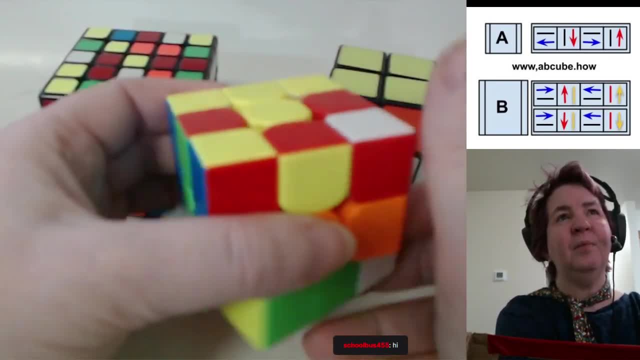 Okay, White's on top, Slide it Out down in up, Out down in up. Okay, White's on top, Slide it out of the way. White's on top, Slide it out of the way. 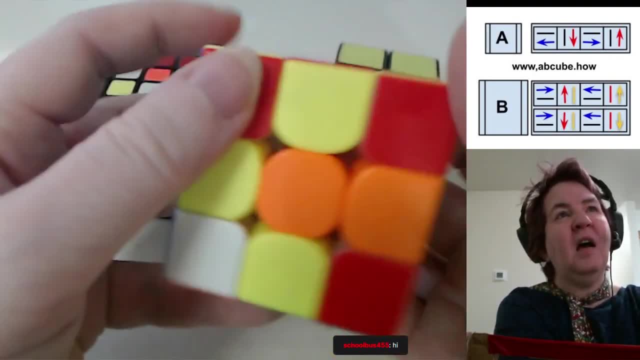 This one can still be twisted. So out down in, up, Out down in, up, Out, down, in up, Formula A until the white comes to the top. And now we can check, and our yellows are still happy. 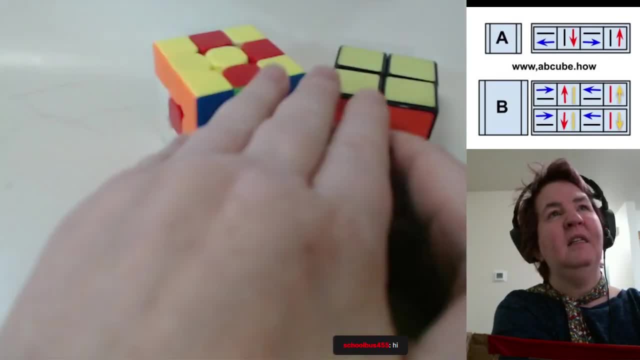 They're still where they're supposed to be and correct to each other. Okay, So we brought the white to the top. Let's do it on this one. Yellow face down. Okay, White's on top. Slide it, Rotate the top. 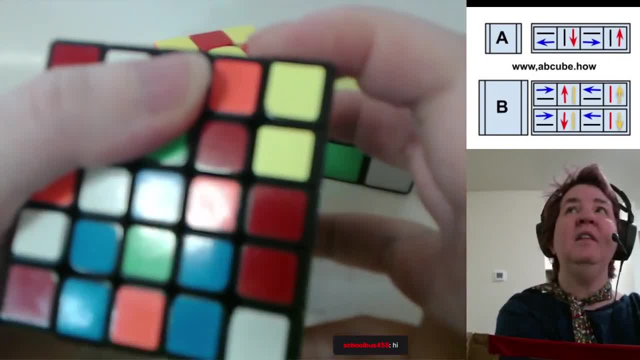 Out down in up. Out down in up. Okay. White's on top. Slide it out of the way. White's on top- Okay. So we brought the white to the top. Let's do it on this one. 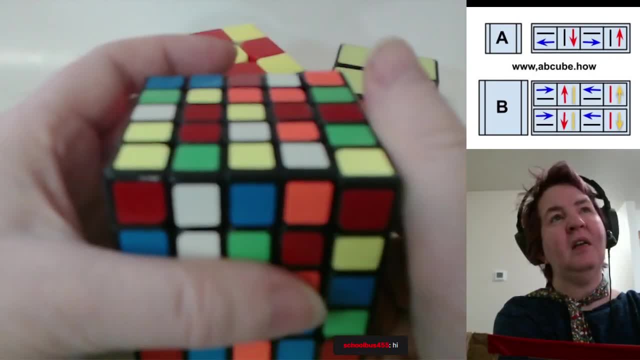 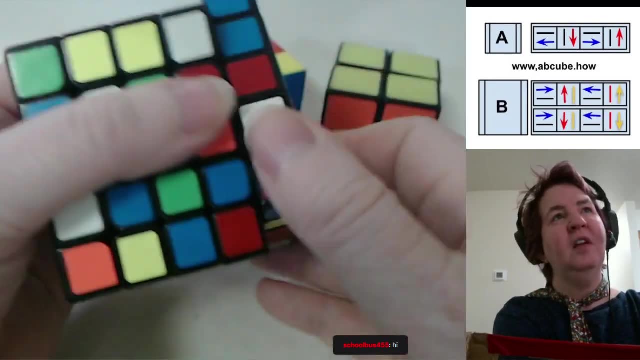 Yellow face down. Start with one that's already white, if there is one, And Formula A to twist this cube until the white's on top. It's multiple of two, because it goes down and then it comes back up again. White's on top. 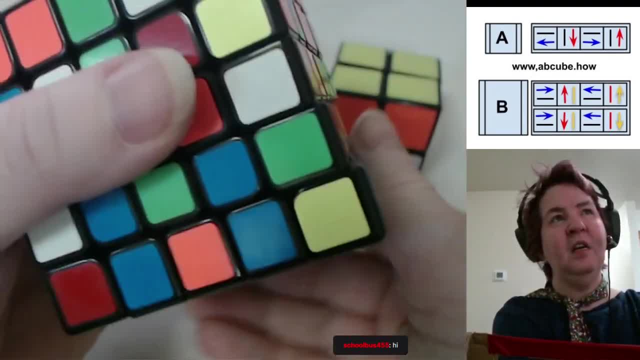 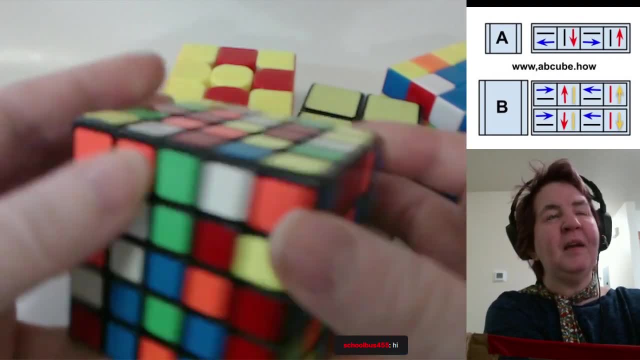 Hold the cube stable, Twist it out of the way. Top row only. Continue with this one. Formula A: And yes, we can see that the yellow's dancing around, but we're ignoring it. yellow Until we get the white on top on all four corners. 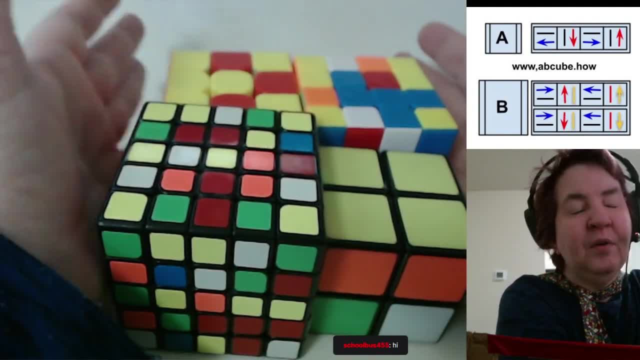 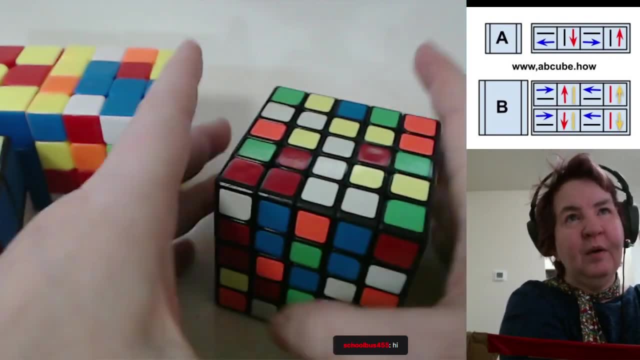 And now the yellow has resolved itself, Resolved, resolved, Okay. So white's on top here. White's on top here. White's on top here. Yellows are still happy. Yellow face down. Here's a white. 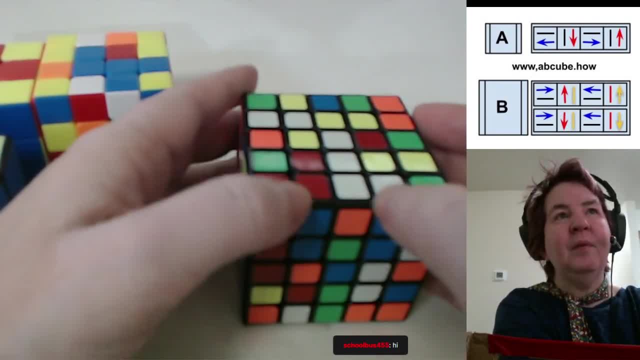 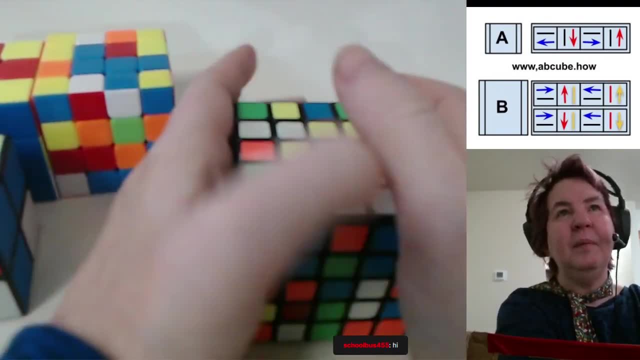 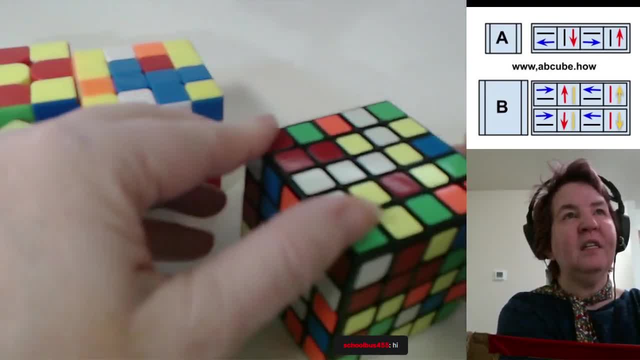 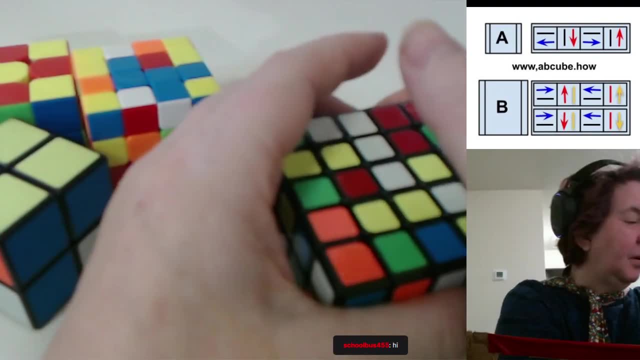 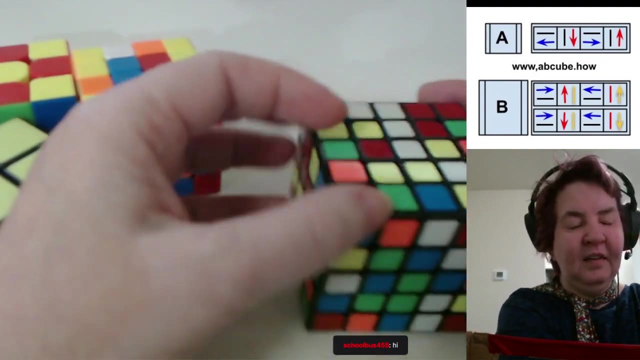 Out down, in up, Slide the top. Formula A, Until the white's on top, We're ignoring the yellows, even though we can see that they're dancing around. And when the white's on top, the yellows are back in where they're supposed to be. 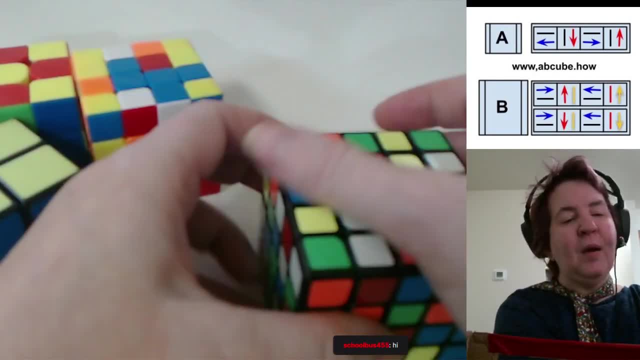 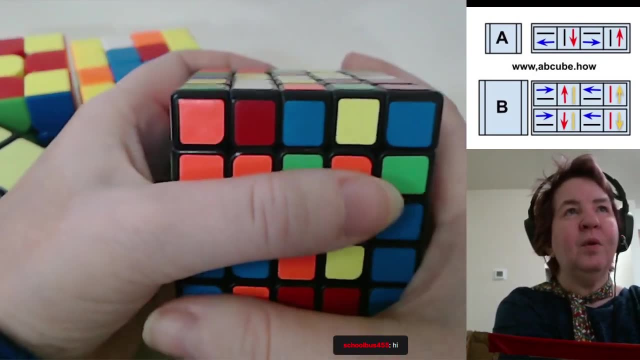 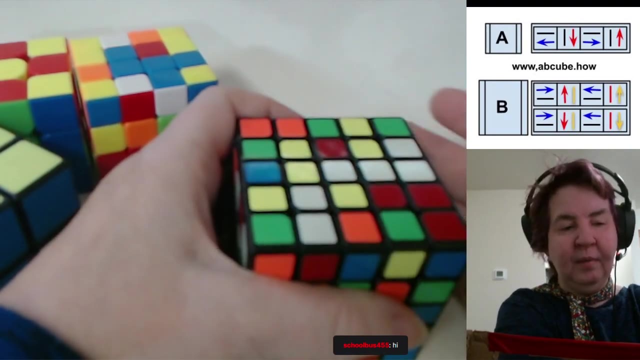 Okay, Okay, Is anyone joining? Good morning If you've just joined me. I am Sunshine And we're working on cubes this week, As we should. Our yellow. we're working on corners. Our yellows are done. 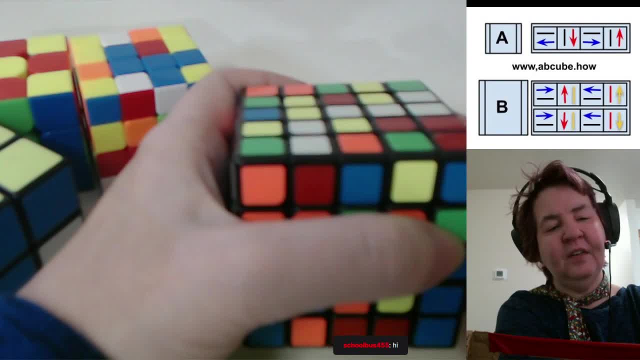 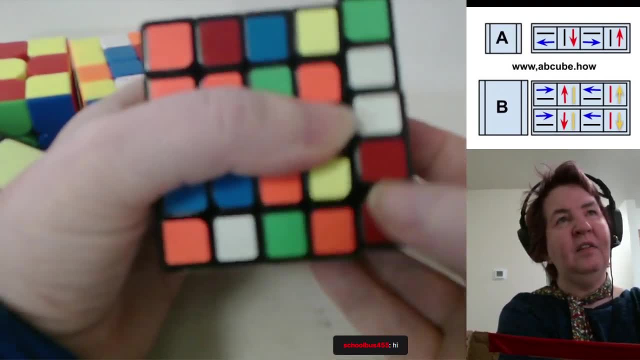 We've got the white to the top color Now, same as with the first four corners. at this point in time, one of three things has happened With the white on top. looking at the side colors of the corners, either all four sides- 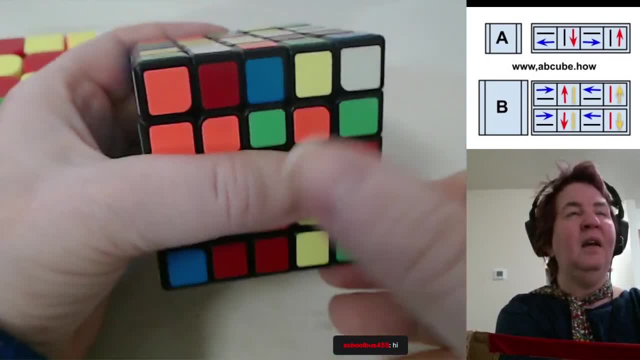 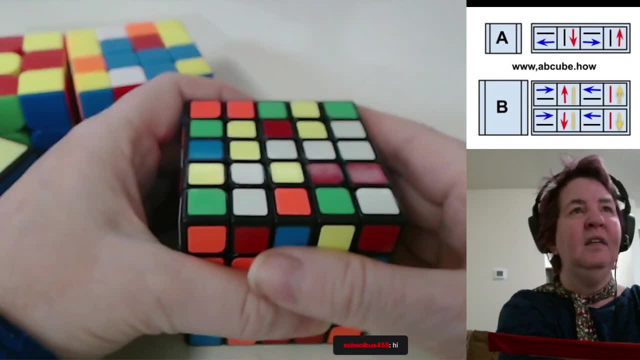 sides match to each other. None of the four sides match to each other or one side matches. You can't have it any other way unless you've been peeling stickers off. Don't peel stickers off. Don't peel stickers off. Okay, So this one orange equals orange. Green does not. 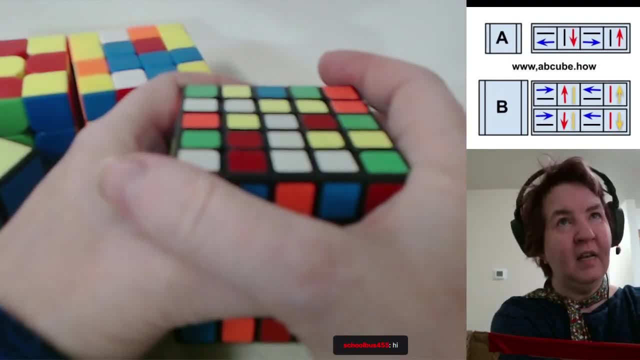 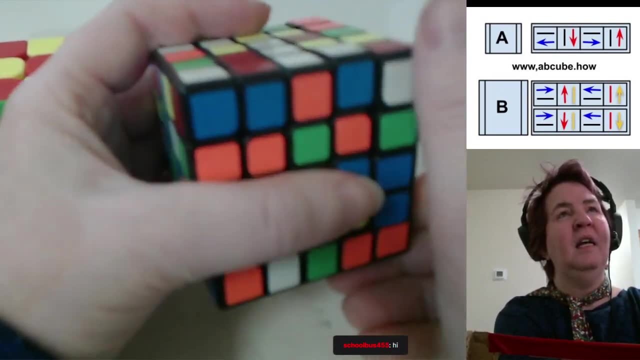 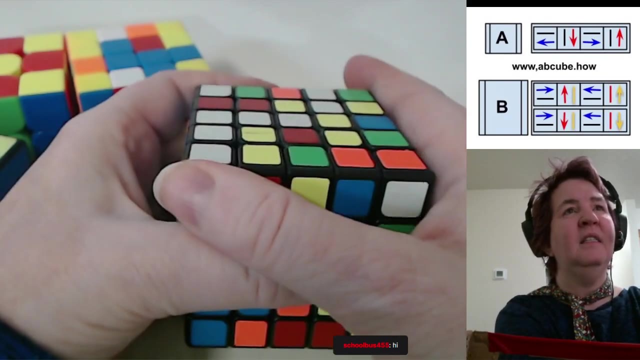 equal red. Blue does not equal green, Red does not equal blue, So this one has one side. This one. green does not equal red. Blue does not equal green, So this one has one side. This one, one side. Most of the time you'll have one side, but sometimes you won't, So 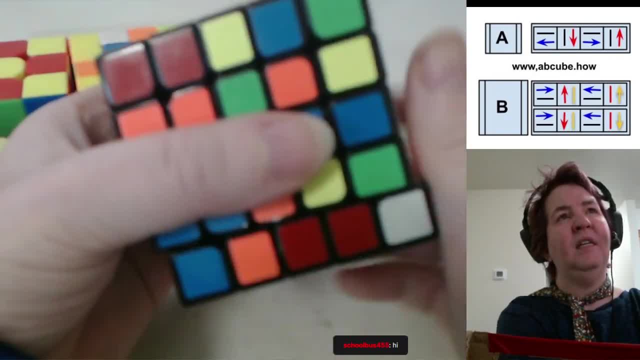 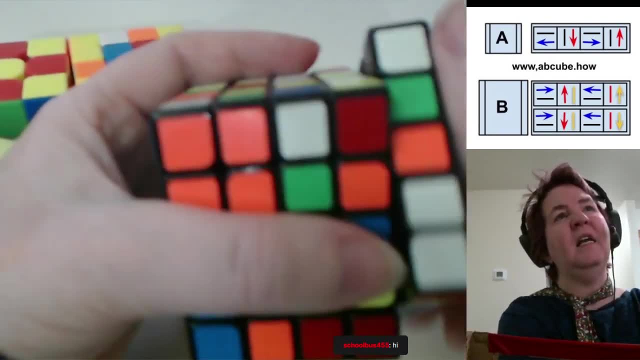 this one. red does not equal orange, Blue does not equal green, Red does not equal orange, Blue does not equal green. So if none of the sides are correct, it doesn't matter which way you hold it to begin with. If there is one side, you hold it to begin with.